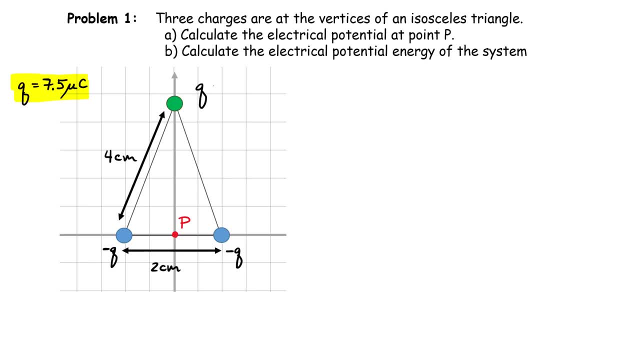 what is the potential energy of the system? So two different quantities that were asked to calculate. So for the first one, how do you calculate the total potential V over at point P? So if there's three charges, remember you need to know the magnitude of the charge and you need to know the 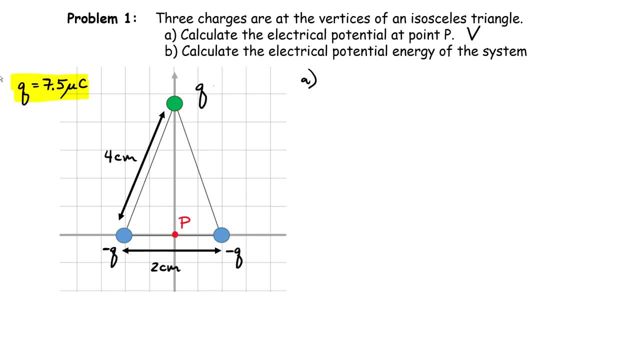 distance to the point where I'm evaluating it. So for this I'm going to use a conservation of energy at point P. So I'm going to use a conservation of energy at point P. So for this arrangement I've given you that the top charge is positive and these blue charges are minus Q, same magnitude but different. 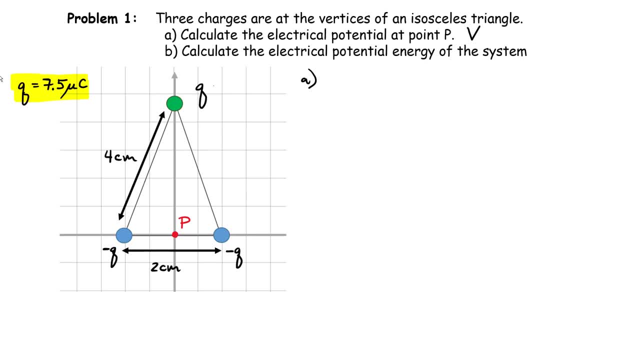 sign from the green one, And each charge here has a magnitude of 7.5 microcoulomb. So let's go ahead and just define some distances here. So I'm going to define this distance, which is going to be the same as the other one, but just to keep it neat here we're going to call this B And I'm going 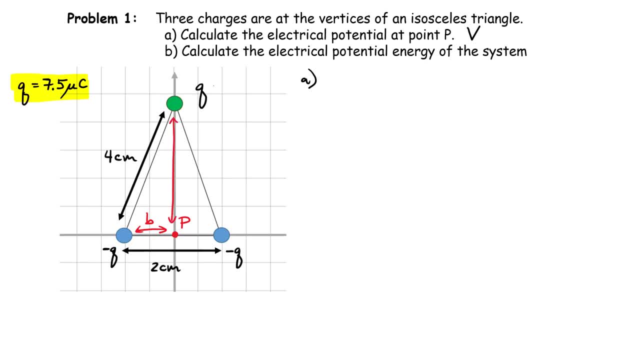 to call the distance here from the top charge to the point P. I'm going to call that A because now you can see I have a distance of 7.5 microcoulomb. So I'm going to call that B and I'm going to call. 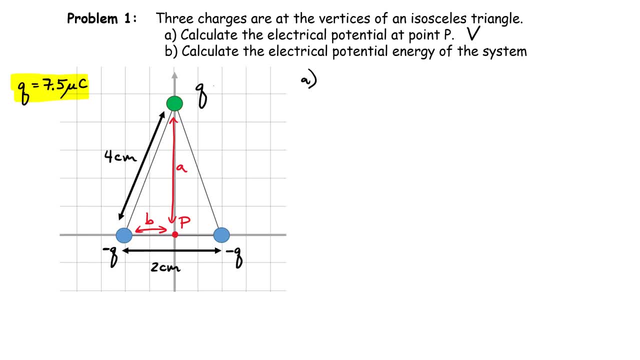 that B, and I'm going to call that B because now you can see, I have a right angle triangle, I can calculate these distances Because right away you should know that the value B must be equal to one centimeter. Okay, How would I find the value A, for example? Well, now you just use Pythagorean, right, You would? 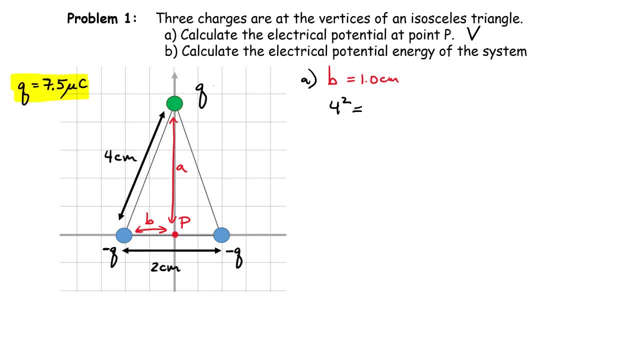 say that the hypotenuse 4 squared has to be equal to A squared plus B squared, And B, I know, is 1.. So that means that A would have to be the square root of 4 squared minus 1 squared. 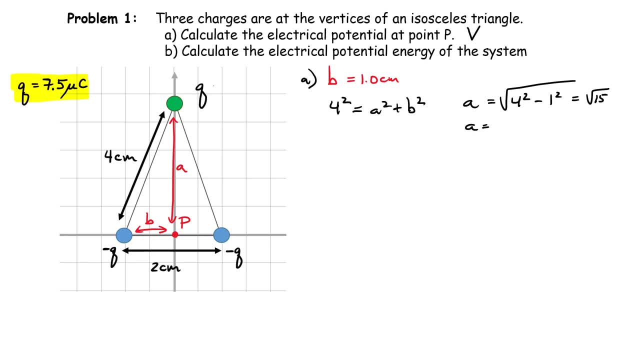 Which gives me square root of 15.. Put that in a calculator. I think you should get something that's around 3.87, again measured in centimeters. All right, So I think now we're in a position where we can calculate the total electrical potential. So the way that I calculate V total is just simply. 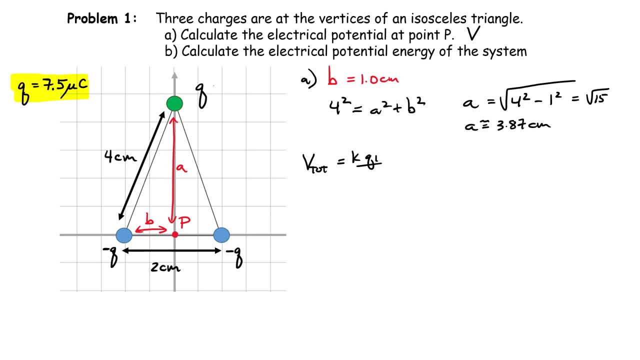 K, Q1 over the distance over here. I'm going to call that, say, R1. for now, Let's just write down a general equation and we'll substitute in all our values. So let's just write down a general equation. 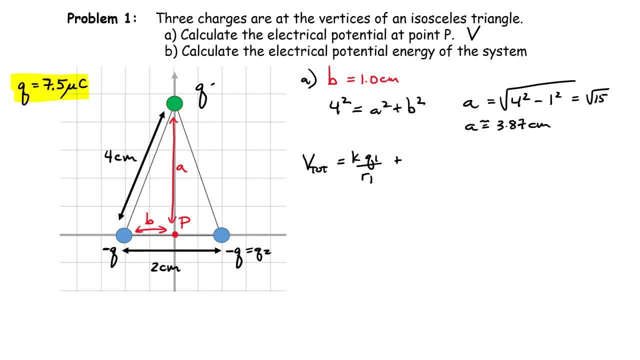 Q2 will be this one, And Q3, I'll call this last one over here. So I have three contributions over here, right? R2 plus KQ3R3.. All right, Now we're going to use some of these variables here. that. 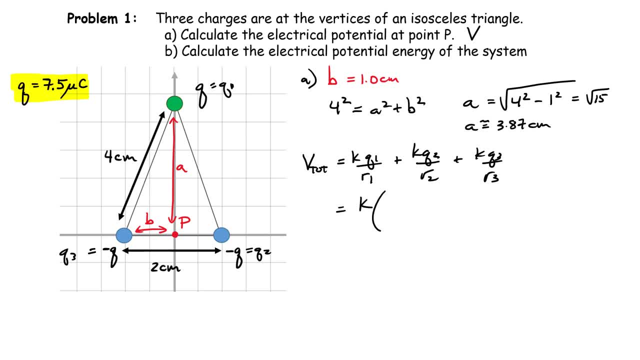 I've introduced. I can factor out that constant K, because it's the same for all three. All right, The value of Q1 is simply Q. right, I'll just put it in as Q. All right, So that is going to be this distance A that I just solved for. All right, What else Plus? 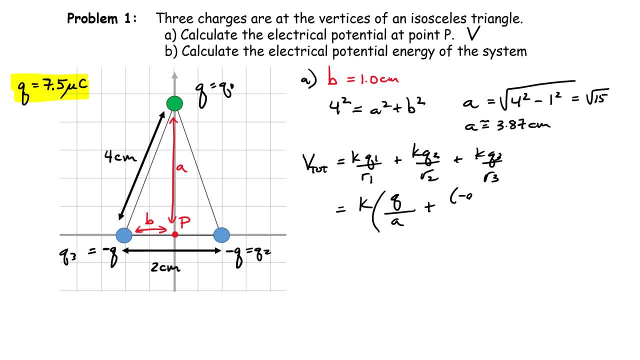 what's the second charge? The second charge here has a magnitude of minus Q. You have to put the sign here when you calculate potential, because it's a scalar quantity. The distance to the point is also B, that one centimeter value Plus. what's the last one? The last one here is also minus Q. 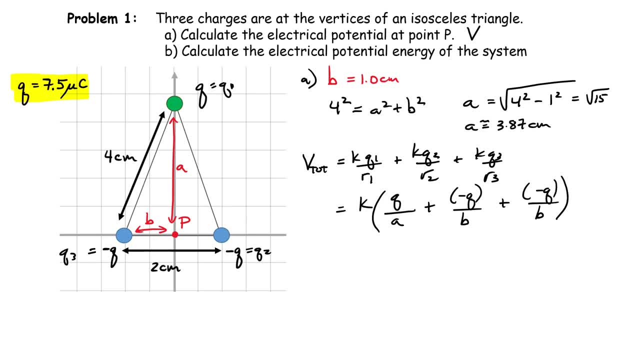 And again, it's also a distance of B away. All right, So guess what You can combine both of these last two terms and you'll get the distance of B. All right, So guess what You can combine both of these terms to make your life a little bit easier. All right, So what do you get? Q over A? 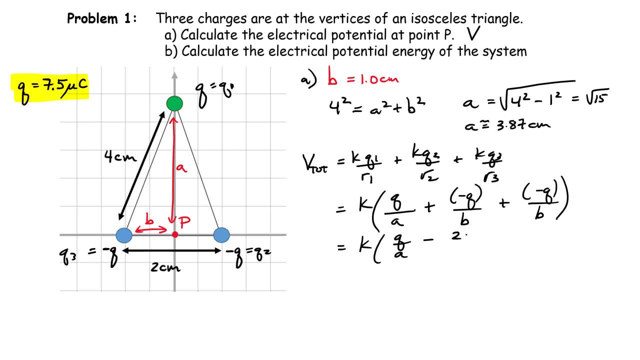 and then what Minus 2Q over B? All right, I kind of like to do this. I'll substitute the numbers at the very last step. I'll also take out the value Q and I'll bring that to the front. So we. 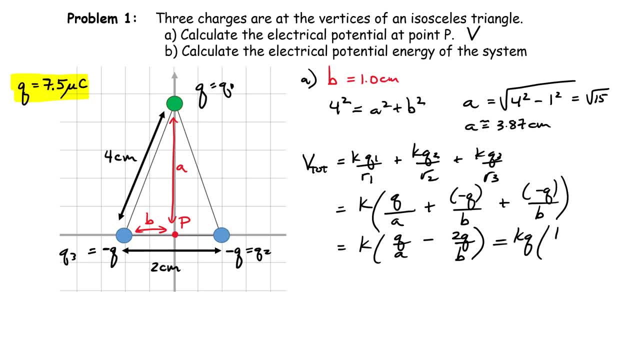 have KQ. So that way it simplifies some of the numbers that I have to substitute in here: Minus 2 over B. Okay, So that's the value or that's the expression for V total, And now I'm just going to substitute everything into the calculator. So, 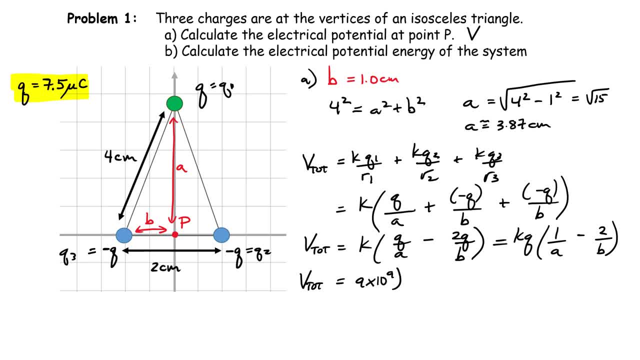 for K I have 9 times 10 to the 9.. What else? Q was my 7.5.. Now it's in microcoulombs, So that's 10 to the minus 6.. All right, So now we have to substitute our numbers. It's 1 divided by A. 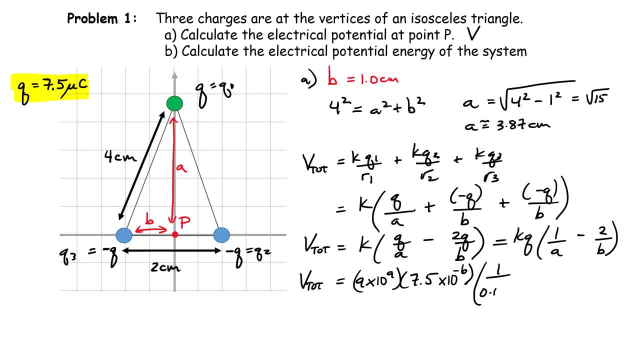 A was 3.87 centimeters, But again, I want to convert that to meters. Okay, And then minus 2 over B. B was 1 centimeter 0.01.. All right, If you put everything in the calculator and you're. 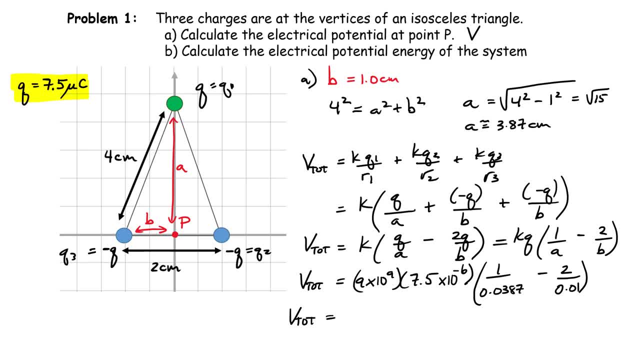 careful with all of these exponents. I think I had something like minus 11.76.. If I round multiply times 10 to the 6 volts, Now you can convert that to megavolts if you want, but that's a lot of voltage, right? Okay, And that's the value for the electrical potential. 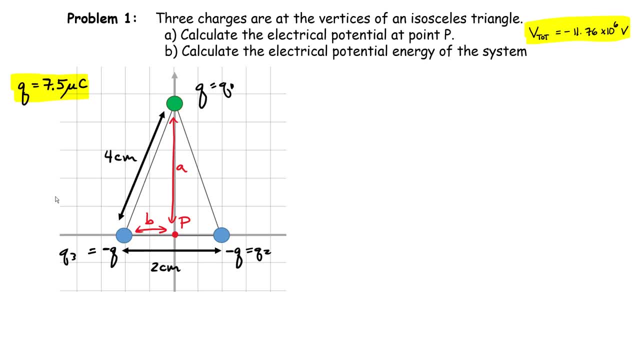 at point P, All right. Second question says: calculate the electrical potential at point P, Potential energy now, of this entire system. All right. So to calculate the total potential energy, what you have to do is you have to consider all the pairs. Okay, So this is what. 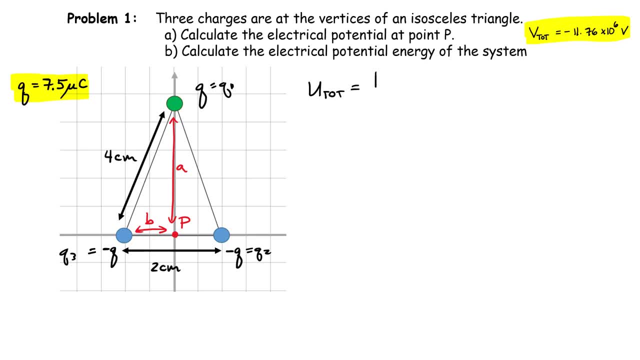 it would look like. So we have. actually, I'm going to call this right- U12.. That's the interaction between Q1 and Q2, plus the potential energy now between the charge 1 and 3.. Call that 1, 3.. And plus the potential energy now between the blue charges. We're going to call that 1, 3.. 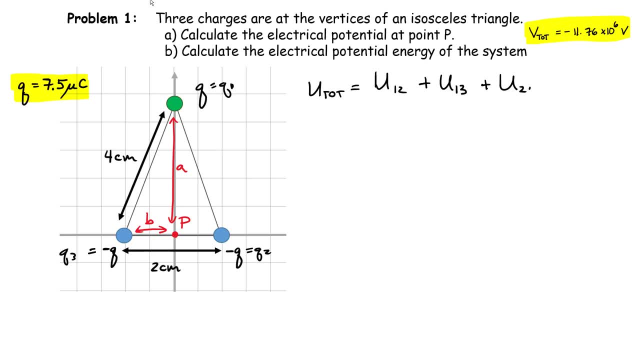 Call that 2, 3.. Oops, All right. Now for each pair we can substitute the equation. It looks similar to the potential, but keep in mind there's two charges here: right Q1, Q2, divided by the. 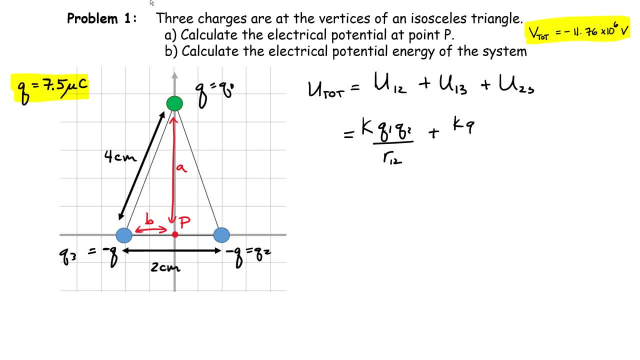 distance between 1 and 2.. Plus K Q1, Q3 divided by the distance between 1 and 3.. And the last one, K Q2, rather Q3 divided by the distance, now 2, 3.. All right, Now when we're again, this is a scalar quantity. So when you substitute the 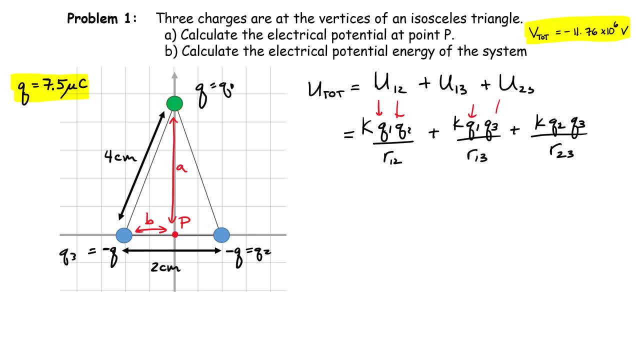 charges. here it's very important to put positives and negatives. if the charges are positives or negatives, All right. Now let's go ahead and substitute. We can again factor out the K constant That's common within each one. Let's look at the interaction between 1 and 2.. So we've 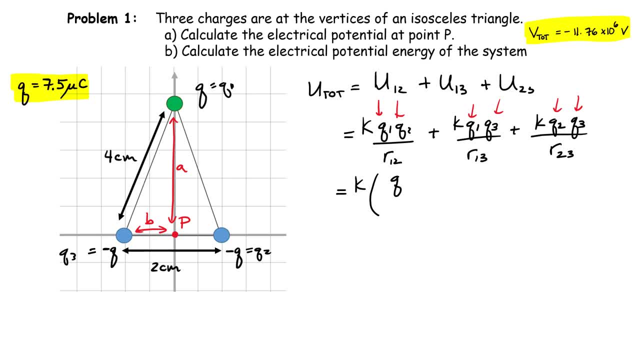 got our first charge, which is going to be positive Q, and our second charge, which is minus Q. All right, These are multiplied by 2.. So we've got our first charge, which is going to be 0.04, divided by the distance. That distance here is this 4 centimeters. Well, let me just go 0.04. 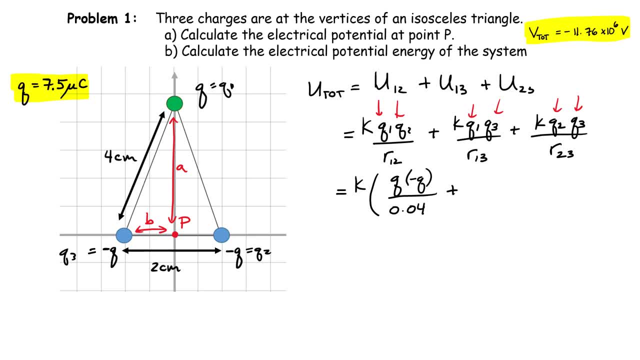 right away, Plus the interaction now between Q1 and Q3. That's this one and that one. So again you get positive Q multiplied by minus Q and the same distance divided by 0.04.. So those first two terms are the same. Now we have the last one, which is Q2, Q3. 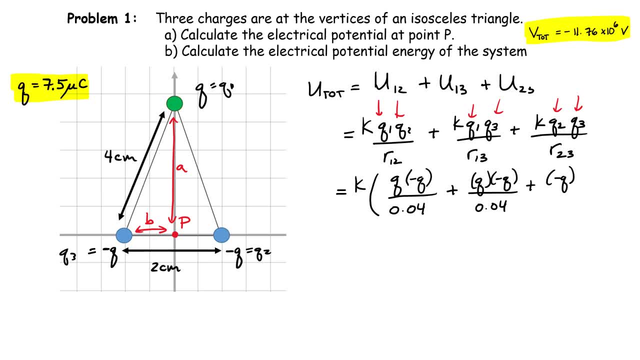 Q2 has a value of minus Q and Q3 has a value of minus Q, And now all that gets divided by our 2 centimeters. Okay, Now let's just take care of some of these positives and negative signs here. So the first one is: minus Q squared over 0.04.. And look, there's two of those terms Actually. 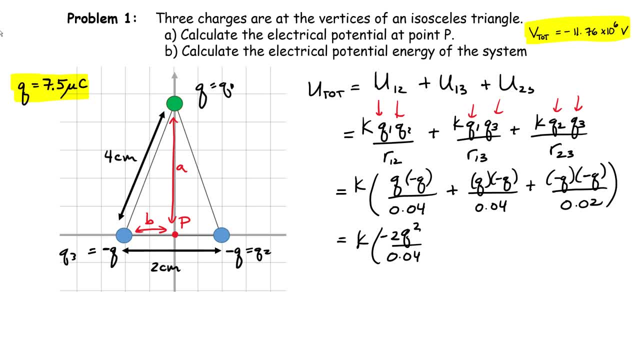 let me give myself a little bit more space. And I'm going to put minus 2.. I'm going to combine both of those terms into 1.04.. And I'm going to put minus 2.. And I'm going to put minus 2.. And I'm 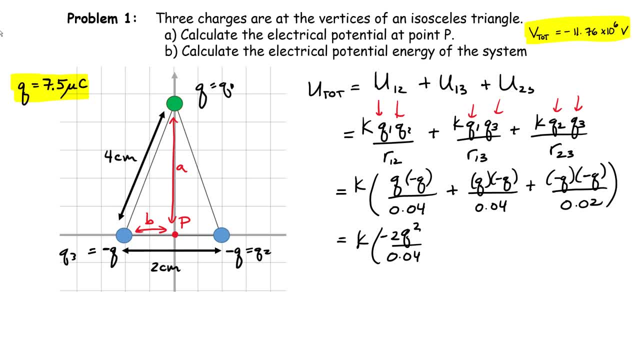 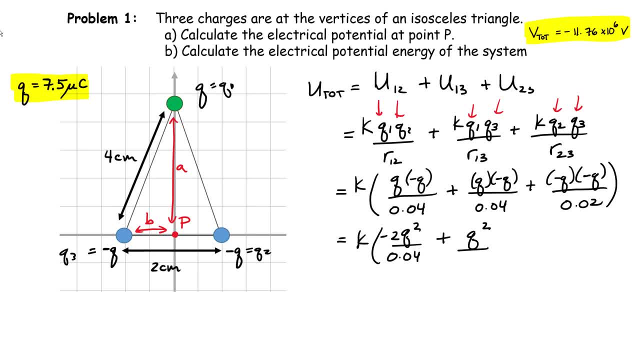 those negative charges, you're going to get Q squared over 0.02.. All right, my last little bit of algebra here. I'm just going to factor out the Q squared before I substitute the numbers, And I get minus 2 over 0.04 and plus 1 over 0.02.. Now, this might not look obvious to you. 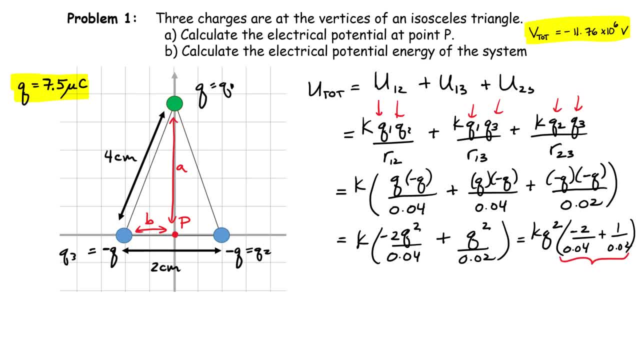 but this guy right here. it just so happens for these three charges- and this is just a coincidence because of the values of the distance and everything else that I picked- that this here actually will cancel out and give to zero, because the first term's negative and it's positive over. 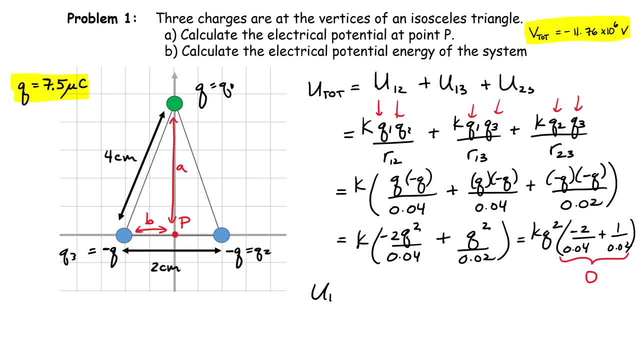 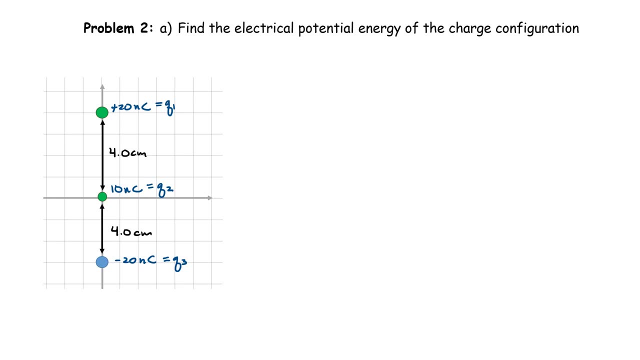 here. So actually for this system right here, the total potential energy is zero joules. There's nothing wrong with that, okay. Potential energy can be a positive, can be a negative value of a system. It could also be zero, All right. problem two says: find the electrical potential energy. okay, Just similar to what we. 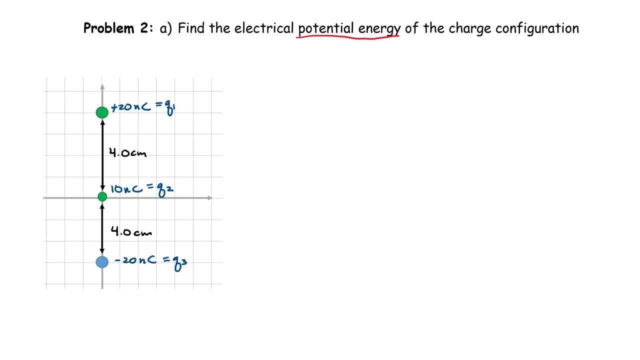 just did for this charge configuration. So I've got three charges here: a 20 nanocoulomb, 10 nanocoulomb and a minus 20 nanocoulomb. I've labeled them Q1,, Q2, and Q3, and you're given. 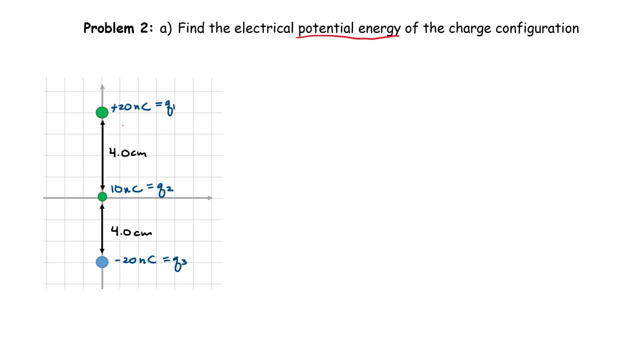 these distances here between the charges. So what we're going to do here is we're going to calculate the potential energy. We need to know the potential energy between every pair. So we're going to do that here. So we're going to do that here. So we're going to do that here. 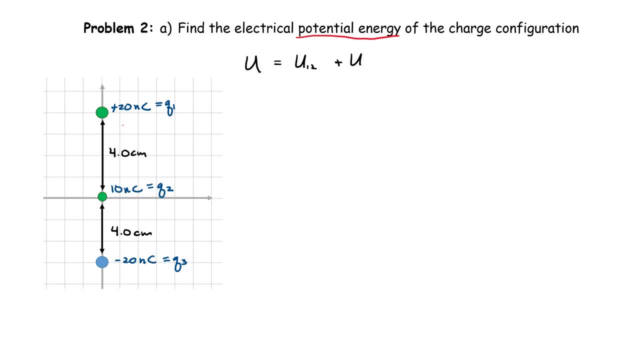 I need the potential energy between one, two, between two and three, and also between one and three. Okay, next step, use the equation for the potential energy between two charges. So here you'd have KQ1Q2 divided by the distance between those two charges, plus KQ2Q3 divided by that. 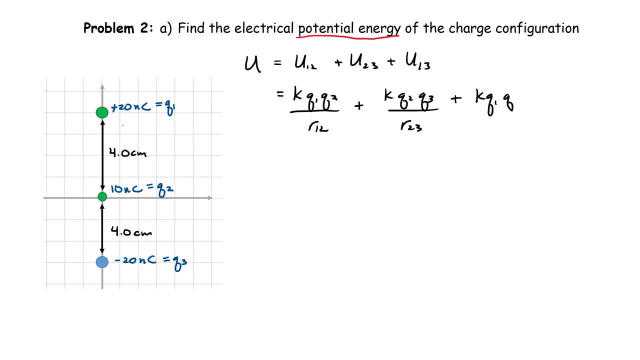 distance and the last one, KQ1Q3, divided by that distance. Okay, next step, start substituting our numbers. All right, so our K value. again, I'm going to factor it out. right, So it's nine times 10 to the nine. All right, we're going to open up a big 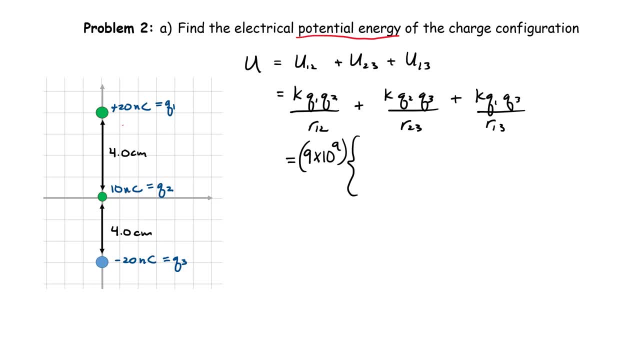 bracket. What I'm left with here are these charges over the distances for the three terms. So Q1 is 20 nanocoulombs. so it's 20 times 10 to the minus nine. Q2 was 10 nanocoulombs, 10 times 10 to the. 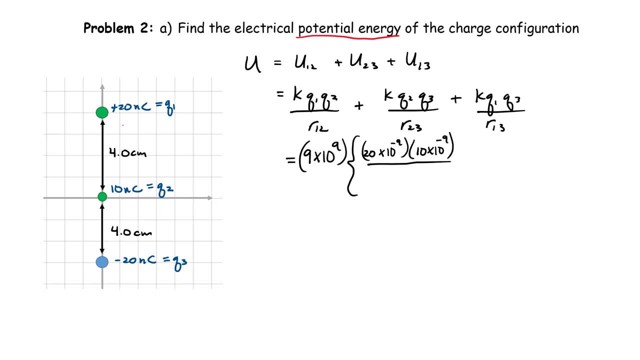 minus nine. Again, you have to put the sign into all of these equations. Now, R12, that's this distance here, that's this four centimeter distance: 0.04, plus Q2Q3.. Q2Q3, we have a 10 and we have a minus 20.. 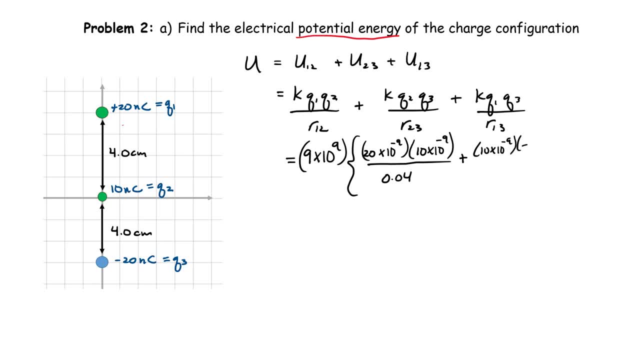 All right, so we have a 10, then a minus 20 nanocoulomb. Now that distance here between two and three is also four centimeters. Now I'm running out of space. I'm going to have to squeeze this in a little bit, And the last one is between one and three. 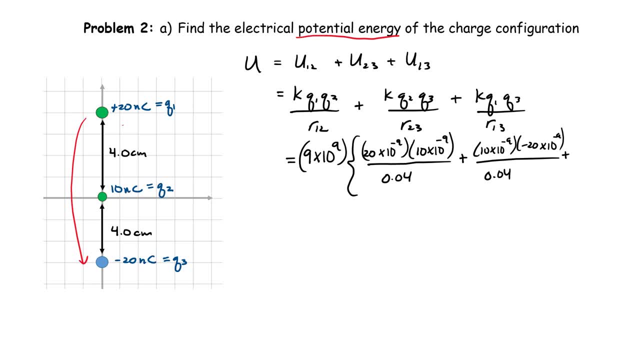 So that's this far distance here, right? So you have to be a little bit careful. One and three is here, So when we substitute, that's a 20 and a minus 20.. Oh, that makes it easier, So, actually, 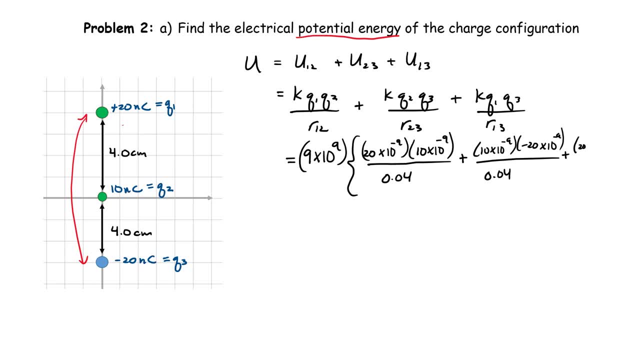 we're going to get. so let's just do 20 nanocoulomb and then a minus 20 nanocoulomb, And all of this now divided by now it's eight centimeters between them, So be a little bit careful- 0.08.. All right, and then you've got to close that final bracket. 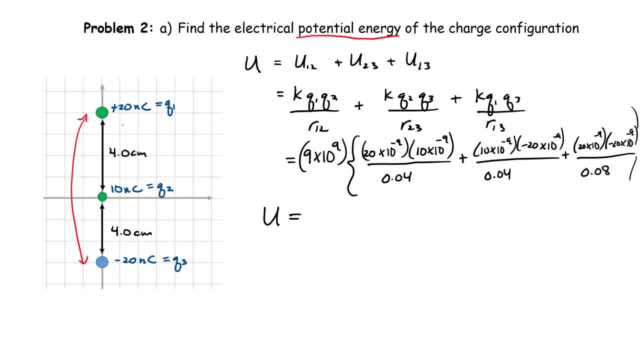 All right, if I put everything in the calculator very careful, what I got here was minus 4.5 times 10 to the minus five. All right, potential energy is measured in joules and that is our answer for part A. All right, let's go look at part B now. okay. 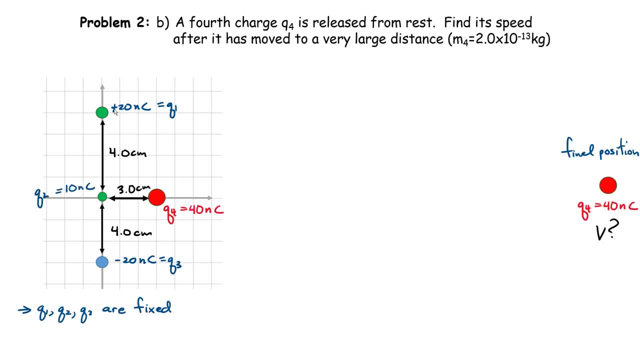 All right, we have now a fourth charge, which has a magnitude of 40 nanocoulomb. It's going to be released from rest. We want to know its speed when it's really really far away. Now we're going to use conservation of. 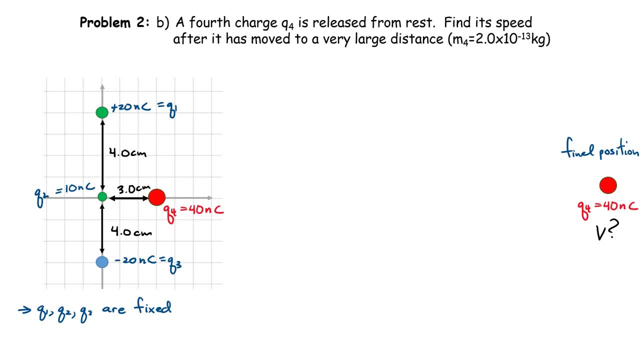 energy for this, okay, And we're going to consider the total energy of the system here and set it equal to the total energy in the final position. So this is what we have. all right, We're going to have the energy of the three charge system. I'm just going to call that mu zero. That's the. 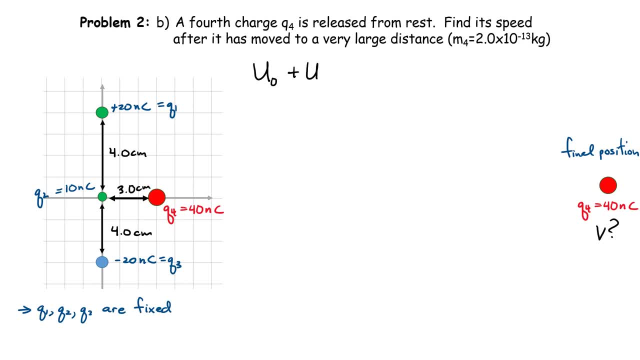 number we just calculated, plus the potential energy of the new charge Q4 that we just added here. okay Now, plus the initial kinetic energy of the system. So this is the total energy initially. okay, This is the number we just calculated from part A And this is the new potential energy now. 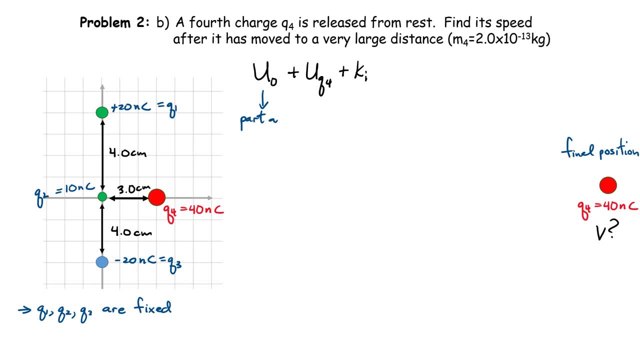 because this guy interacts with the three charges. Now that has to be equal to the total energy in the final position. Now, in the final position, I still have my three charges here, So I still have this U zero. This doesn't change, okay. So a lot of times you don't even include the energy. 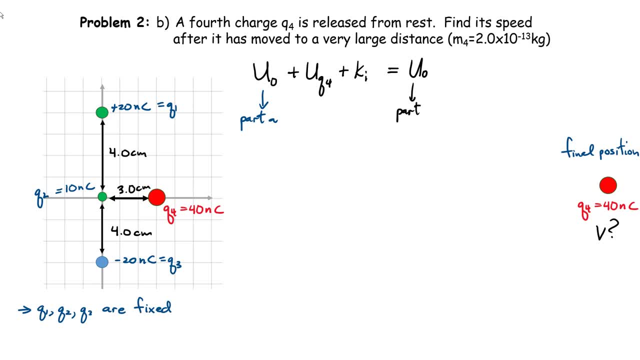 in this part of the calculation. all right, This is the number, part A, that we just did. Now, what else are we going to have? Well, we're going to have the final potential energy of Q4, call it Q4 final- and then plus the final kinetic energy- okay, KF, And it's only Q4 that is moving The. 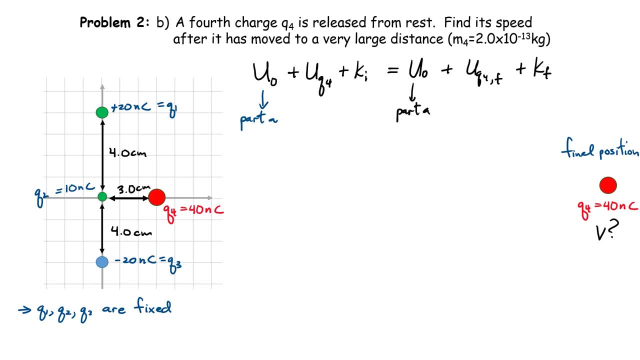 other three charges are assumed to be fixed. Now, since we have this constant term on both sides of the equation, we basically just cancel that out. So we're not really interested in the number of charges, We're just interested in the number we calculated in part A. It doesn't affect anything. 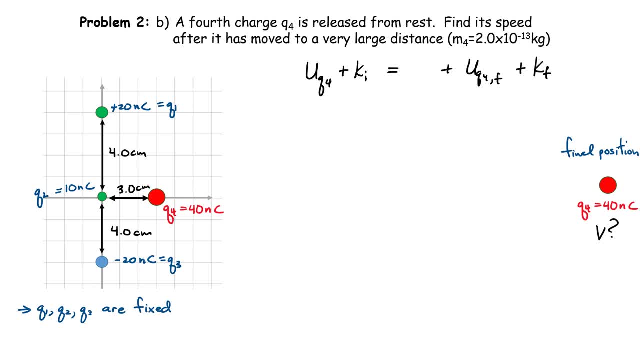 to do with Q4, because the charges are fixed, So that's just the constant value. So this is what we're left with here. We're only looking at the energy associated to that charge, Q4.. Let me move that over Now. we did release the charge from rest So that simplifies this term. There's no. 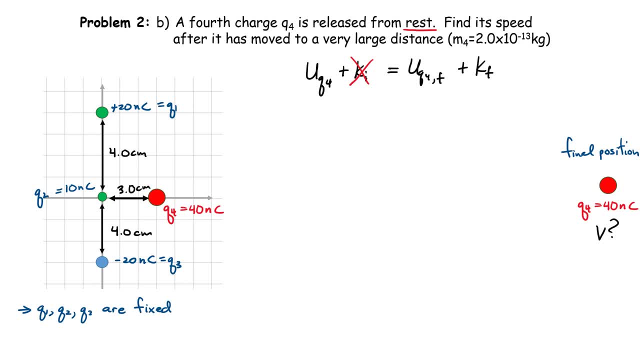 initial kinetic energy. And now there's also another simplification, because they tell us that we're very far away, very large, So we're only looking at the energy associated to that charge- Distances- And what that means is that the value R goes to infinity, basically, And if R goes to 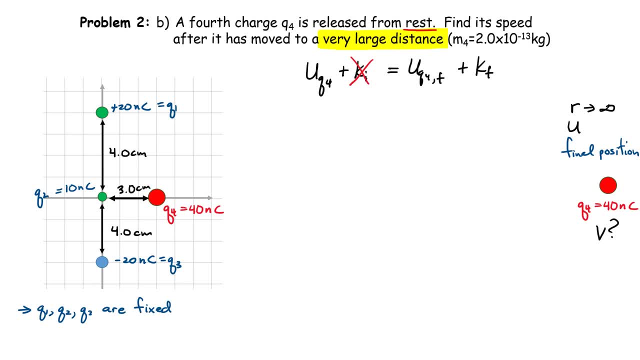 infinity. it basically means that the interaction of Q4 with any of the three other charges. there's basically zero potential energy between them because you'd be dividing by infinity. So we get to eliminate this term when we're very far away. All right, the final kinetic energy, that's. 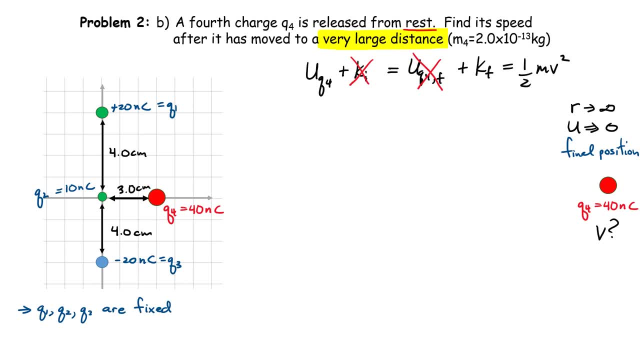 pretty straightforward: It's just one half MV squared. So that is the final kinetic energy And that is where the speed comes in. So all we are left to do now is we need to calculate what is the initial potential energy of this charge in the vicinity of these three other charges. Well, 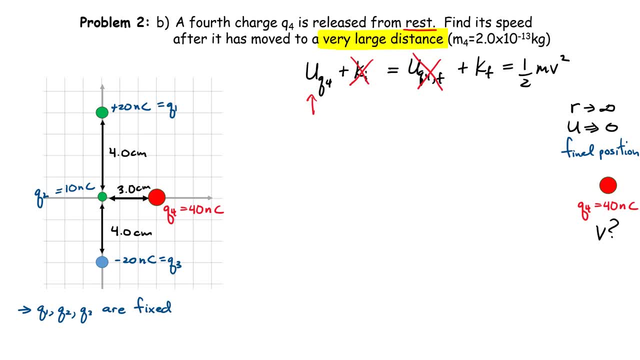 that we know how to do right, And I'm going to do it a slightly different way Now. I'm going to use that the potential energy of any charge you can write as the value of that charge multiplied by the voltage at the position where that charge is located. 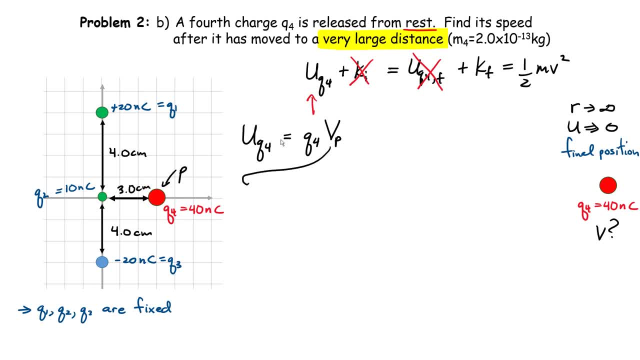 This is the point P. All right, so we first going to calculate what is this electrical potential at this position? And it's the potential produced by the three other charges. Let me factor out that value. okay: Q1 over R1,, Q2 over R2, plus Q3 over R3.. Now we're going to need to know the. 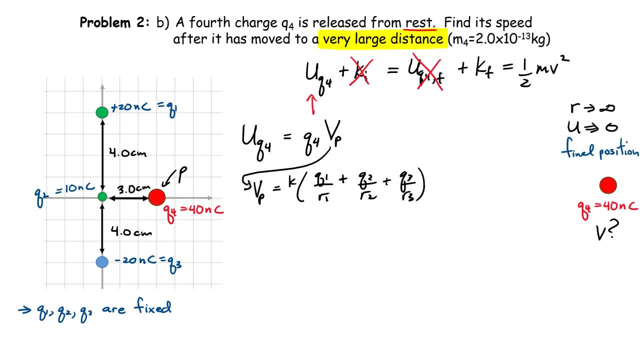 distance between each charge and this point where that charge is located. So if you look at this, we have a triangle over here. This is three centimeters. that's four centimeters. You use Pythagorean theorem, that's five centimeters. All right, now we can start. 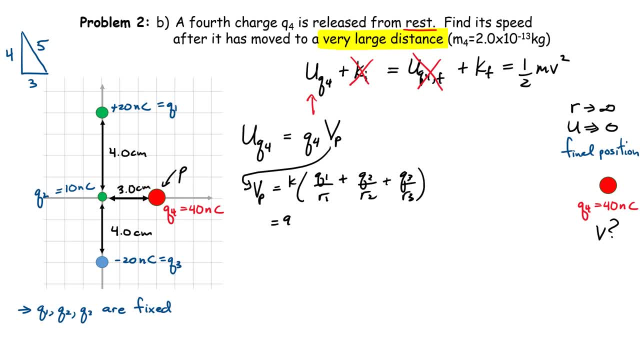 substituting the values in here, right. So we're going to have nine times 10 to the nine multiplied, Q1 was 20 nanocoulombs. 10 to the minus nine divided by the distance, now it's 0.05, five. 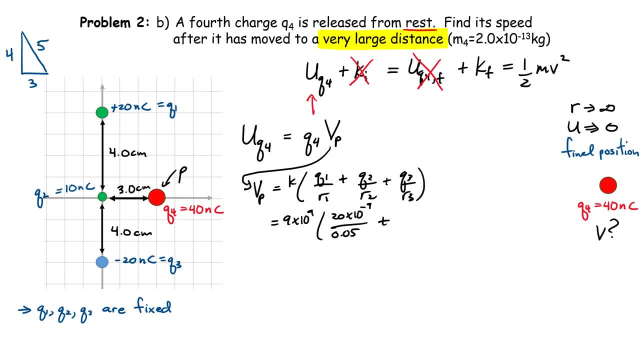 centimeters from that point to where this charge is located, Plus Q2 is 10 times 10 to the minus nine, divided by three in this case. All right, okay. and the last one is a negative charge. It's minus 20 times 10 to the minus nine.